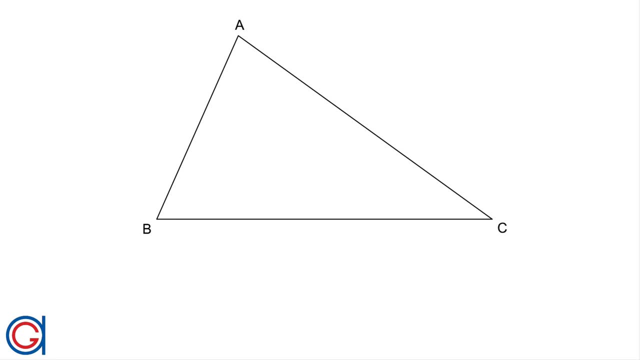 It is located at the intersection point of the angular bisectors of each of the three angles of the triangle. So now to locate this point, we are going to work out the angular bisectors of angles A, B and C of the given triangle. So first of all, setting our compass. 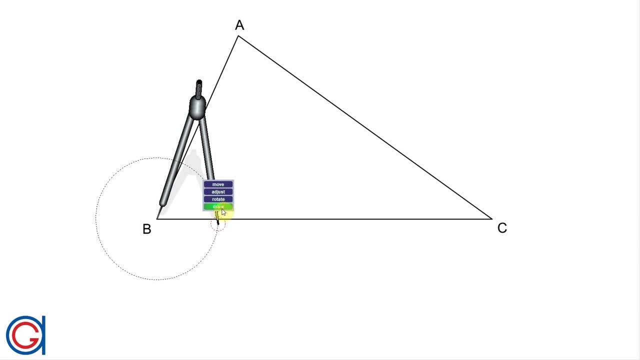 to a certain radius. we set it on angle B and we scribe an arc until it cuts the line segments BC and BA, as shown here and now. with the same radius, we set our compass on the previous intersection point and we scribe another arc, as can be seen here And now. 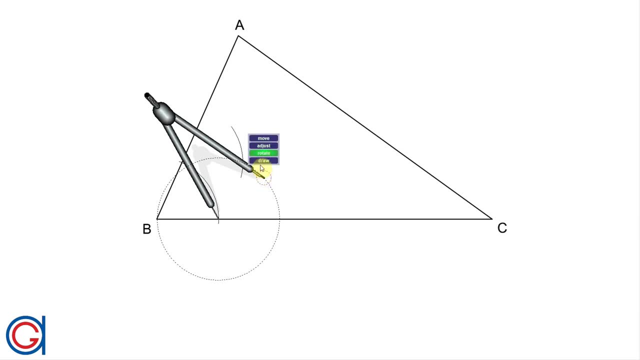 setting the compass. on the other intersection point, We scribe arc to intersect our previously drawn arc. so now to complete our angular bisector, we draw a line from vertex b through this intersection point and we elongate the line, as can be seen here. this is the angular bisector of the angle b. we are now going to repeat this process. 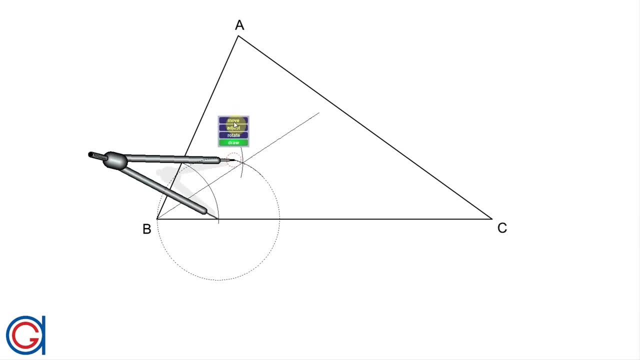 with angles c and angles a. so now again, with the same radius as before, setting our compass on angle c, we scribe an arc until it cuts the other two sides of the triangle, as shown. and with the same radius, setting our compass on the intersection, we scribe an arc. 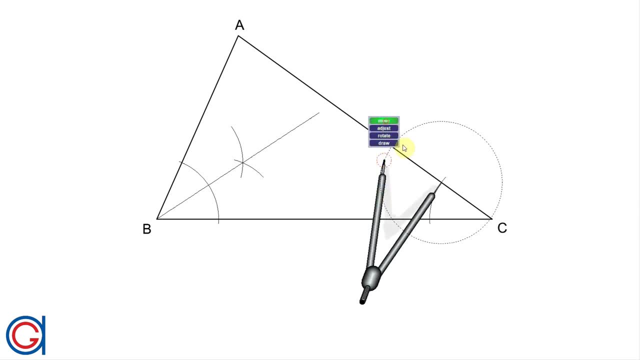 to the left and we cut the other two sides of the triangle as shown, and now, setting the compass on the other intersection point, we scribe another arc to intersect our previously scribed arc and again we join vertex c through this intersection point and elongate the line. 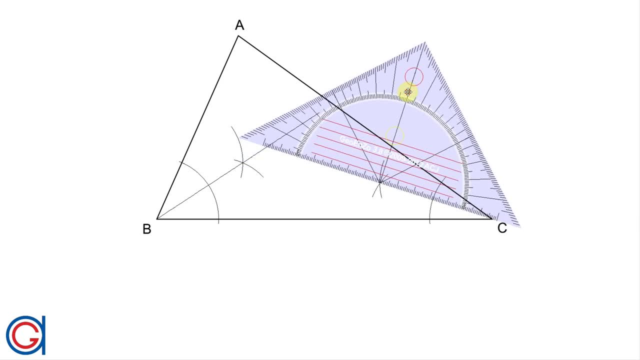 until it cuts our previous angular bisector of the angle b, of the angle b of the angle b. okay, where these lines cross is going to be the in-center point, okay, but just to make sure that we're working with accuracy and precision, we're going to work.